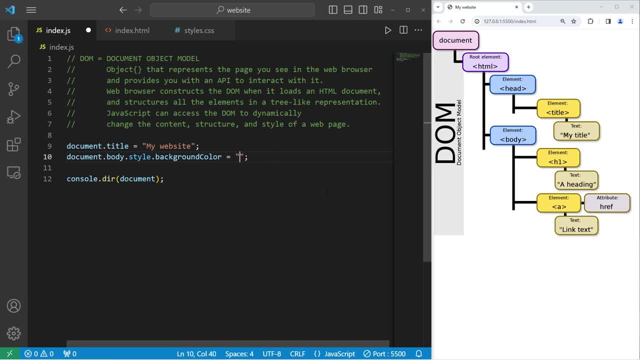 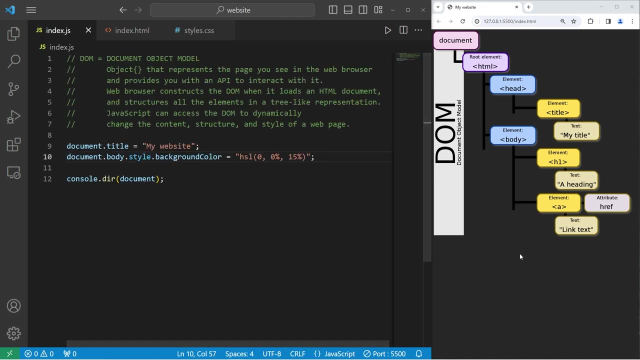 Let's stick with black. for now. I'll use HSL. The hue will be 0.. Saturation will be 0% And the lightness will be 15%. Even though we have no CSS, we're still able to dynamically change the background color. 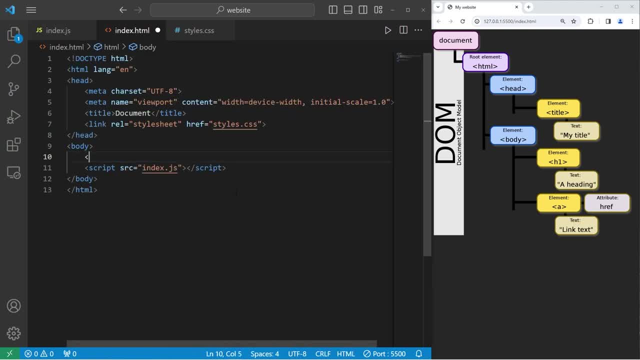 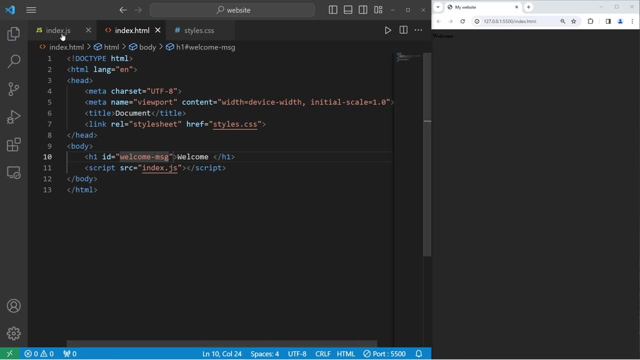 Let me give you another example. We'll create an H1 element. This H1 element will say welcome. I will give this element an ID ID, welcome, DASH MSG, meaning message. And I'm just going to zoom in a little. 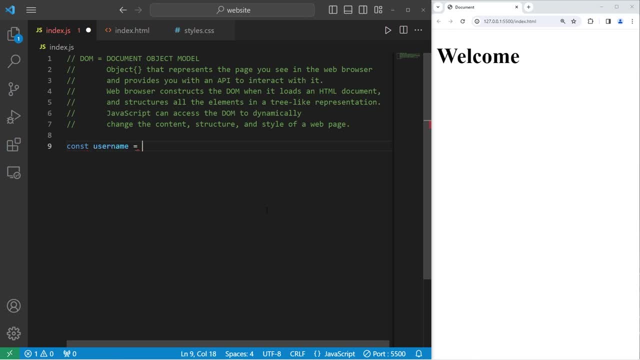 I will create a constant of username Type in your username or your full name. I'm going to conditionally change the content of this HTML document. I will get this element by its ID. Our welcome message. Const. welcome message. Const. welcome message. 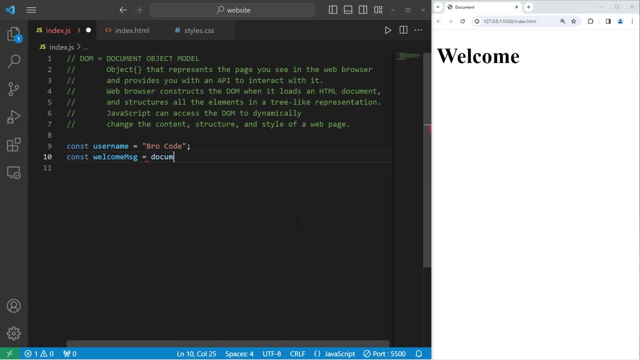 I'm using CamelCaseNamingConvention for this, So I will access my document. use the getElementById method. that id was welcome-message- msg for short. I would like to update the text content of this element. I'll take my welcome message, access the text content of it, then append some text using 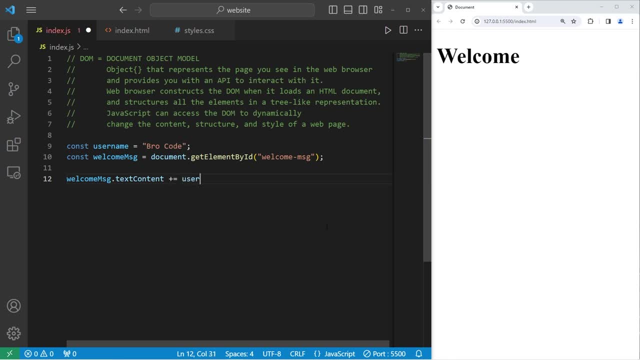 StringCatenation, I'll use the ternary operator to see if my username is strictly equal to an empty string. Is our username empty? Did somebody not type it in? If username is empty, I will append our welcome message with guest. 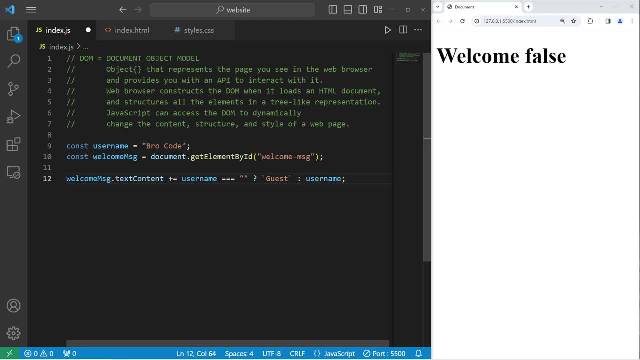 Otherwise, our username, My username, has a name. it's not empty. It will display my name. welcome brocode. If it was empty, if somebody didn't type it in, it will display my name. It will display welcome guest. 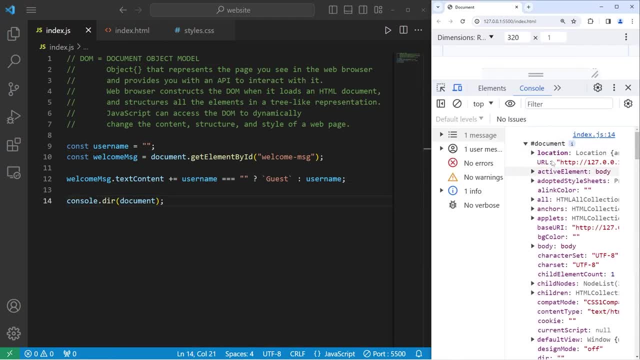 So that's an introduction to the document object model. The document object model is a javascript object that represents the page you see in the web browser and it provides you with an API to interact with it. The web browser constructs the DOM when it loads an HTML document and structures all.